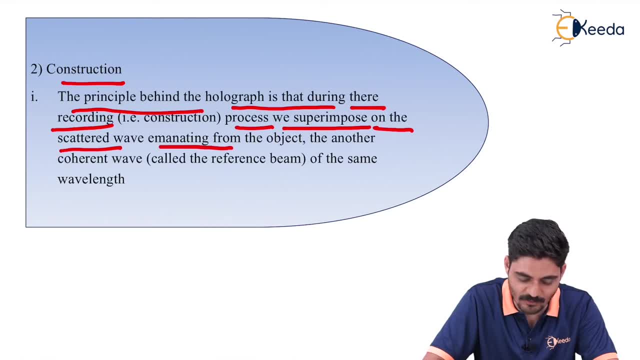 On the scattered wave emanating from the object and another coherent wave of the same wavelength but from laser. So in construction of hologram or holograph, two beams are used. One is the scattered beam from the object of which we are constructing the holograph. 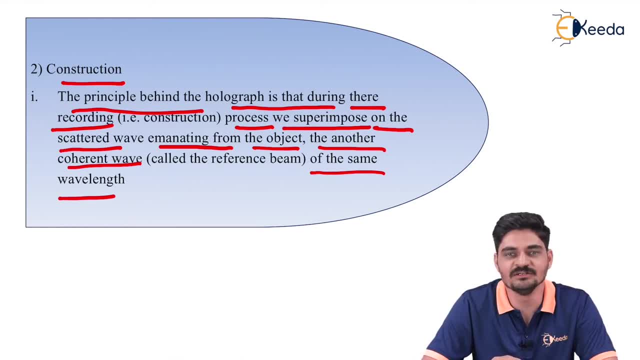 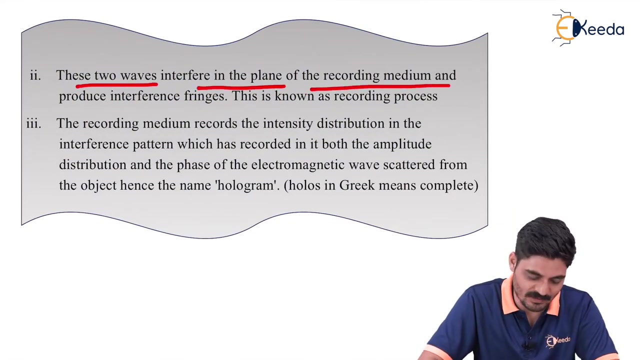 The scattered beam of light emanating from the object of which we are constructing, the hologram, And the reference beam emanating from the laser. So these two beams will be superimposed on a photographic plate. These two waves interfere in the plane of the recording medium and produce interference. 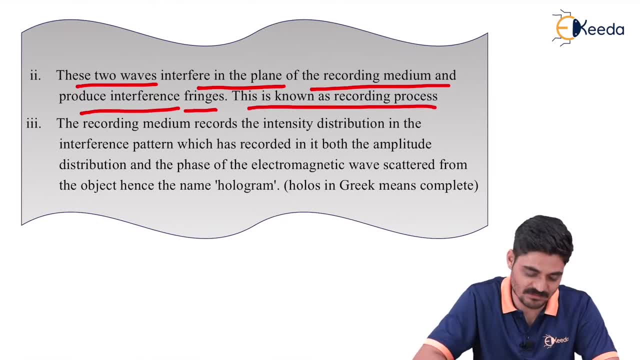 fringes. This is known as recording process. The recording medium records the intensity distribution in the interference pattern, which has recorded in both the amplitude distribution and phase of electromagnetic wave scattered from the object. Hence the name hologram. Here holos means complete. 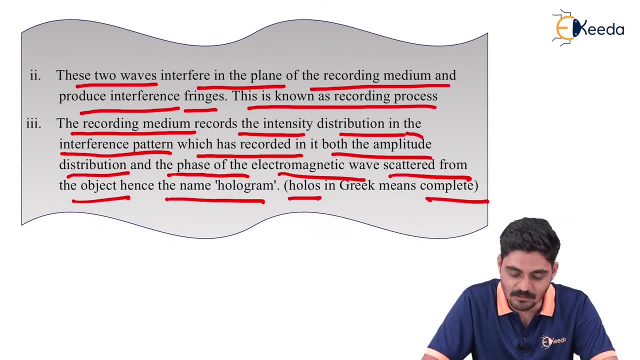 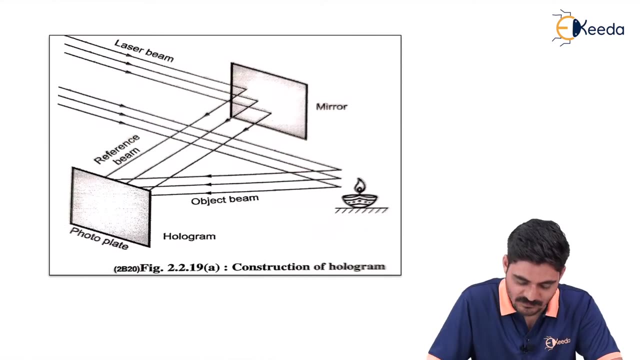 This is the Greek word, Which means complete, And grams or grama means recording. So hologram represents complete recording. This is how the construction of hologram is done Here from this object. Object: beam is incident on photo plate or photographic plate. 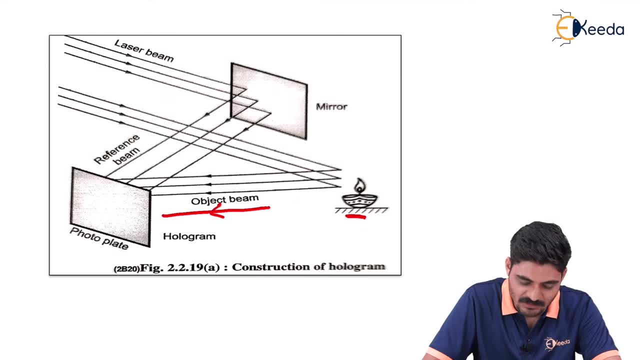 So this is the hologram, This is the hologram, This is the hologram, This is the photographic plate. So this object beam is interfered with this reference beam. This is reference beam. This is coming from laser. So from laser it is first incident on mirror, so that it becomes weak and then mirror reflects. 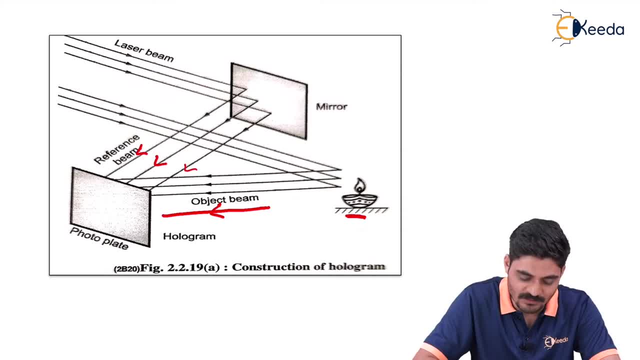 it towards photographic plate. So on photo plate the object beam or beam from the main object to be holographed is incident and while reference beam of laser interferes, it and these two interferes here on photo plate to construct a holograph. So very simple to understand this diagram, Simply taking laser. 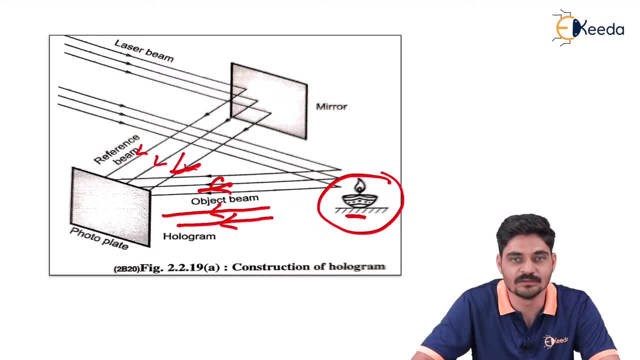 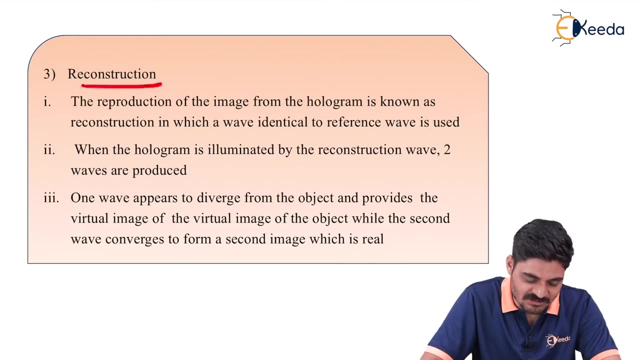 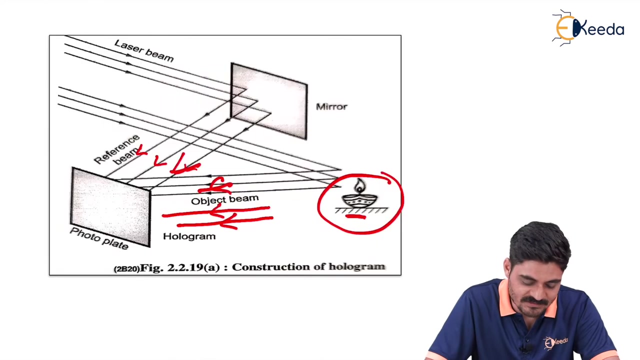 beam to mirror and mirror will reflect it to photo plate and the object, beam from the object will also come to photo plate, and here construction of hologram will be done. Now in reconstruction, the production of the image from hologram is known as reconstruction. See from this diagram. 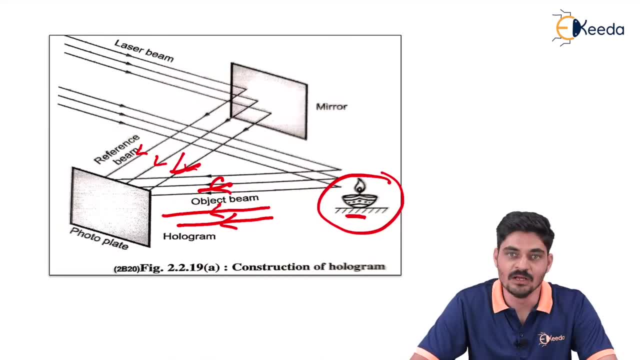 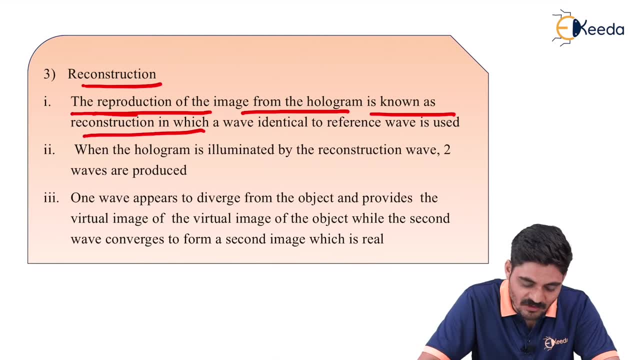 we understood how hologram is created. Now, if you want to reconstruct the image using this hologram, then the production of that image from hologram is known as reconstruction, in which a wave identical to reference wave is used. When the hologram is illuminated by the reconstruction wave, two waves are produced. One wave appears to 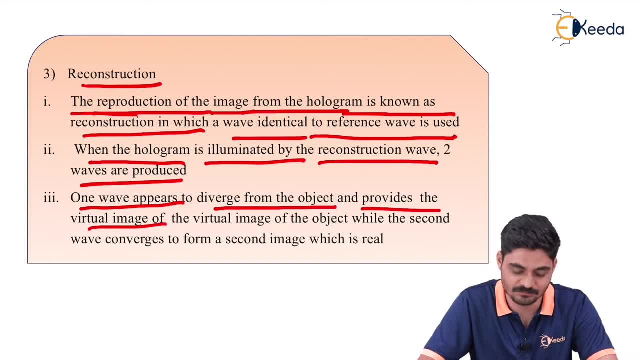 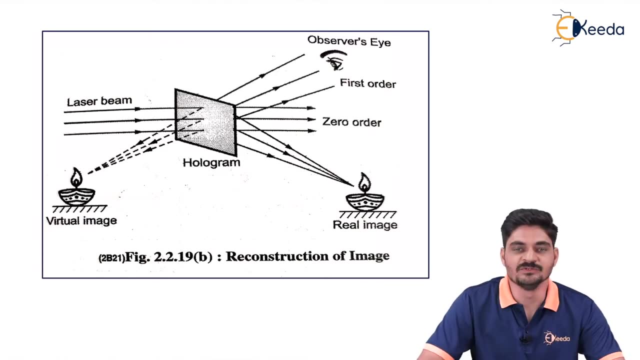 diverge from object and provides the virtual image of the object, while the second wave converges to form a second image which is real, as like shown in this diagram. So in this this is recorded, hologram in which already data is stored, and now we want to reconstruct. 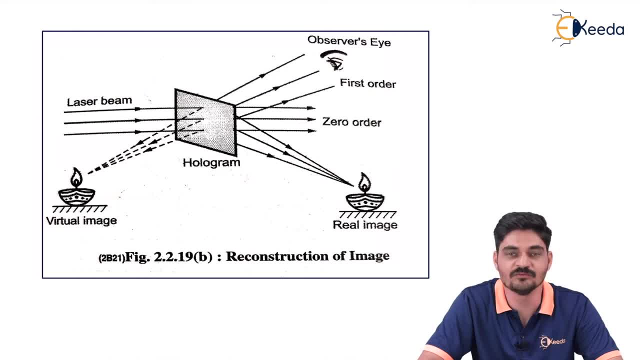 its image. So laser beam will be incident on this. because of that, what happens? a virtual image is produced here and the real image is produced here, and observer will have the complete structure of the object to be observable to it. So this is how reconstruction of image. 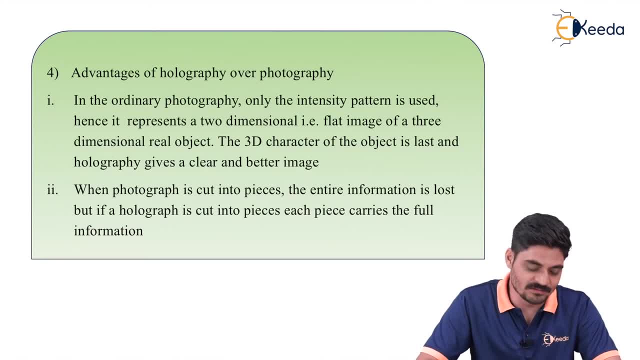 from hologram is done. Now, what are the advantages of holography over photography? Let's understand this. In the ordinary photography, only the intensity pattern is used. Hence it represents only two dimensional or flat image of a three dimensional real object: The 3D character. 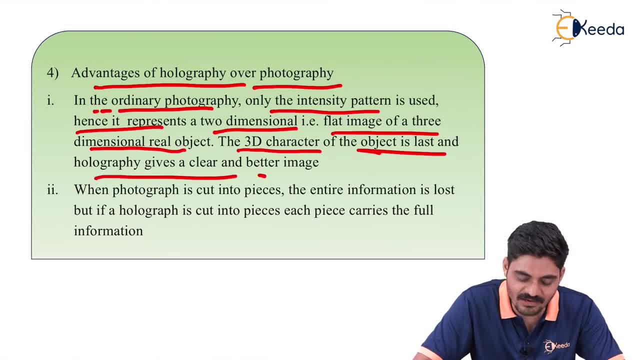 of object is lost and holography gives a clear and better image, because in photography only intensity patterns are recorded, but in holography intensity pattern as well as phase pattern is recorded and in photography we have two dimensional image, while in holography we have three dimensional image. When photograph is cut into pieces, the entire formation is 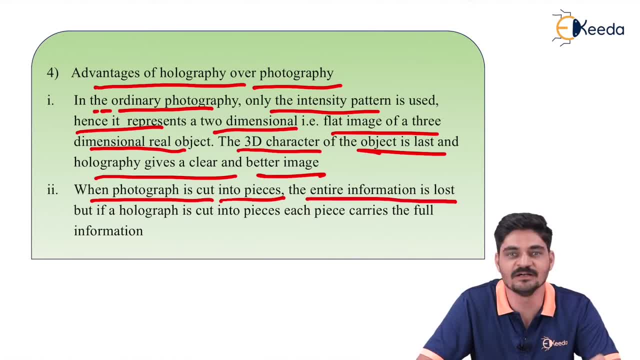 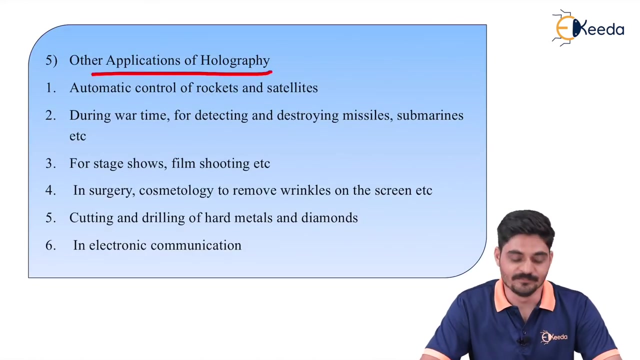 lost. but but the most important advantage of hologram is if holography is cut into pieces, each piece carries the full information and hence entire image of object can be reconstructed from the piece of hologram. also, What are the other applications of holography? Automatic control of rockets and satellites. 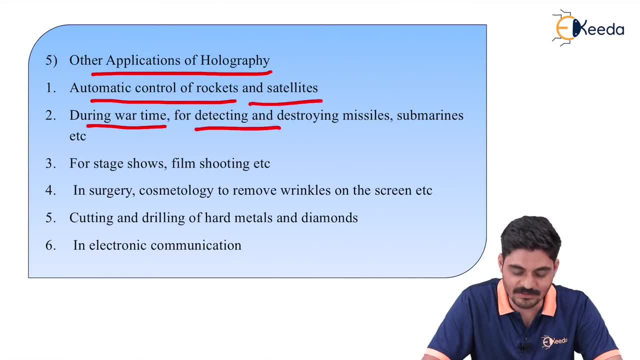 is done by holography During the war time for detecting and destroying missiles, submarines etc. there holography is used: 1. For stage shows and film shootings also. holography is used 2. And in some type of surgery and cosmetology to remove wrinkles on the screen. there also. 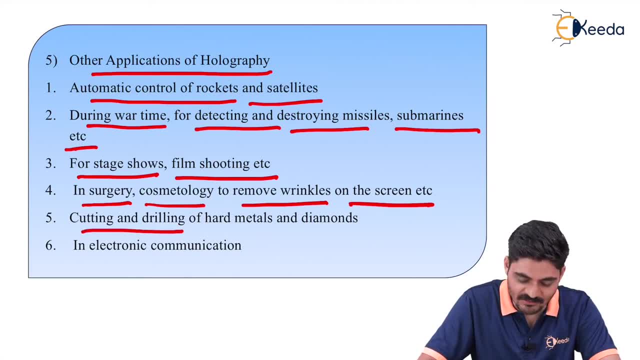 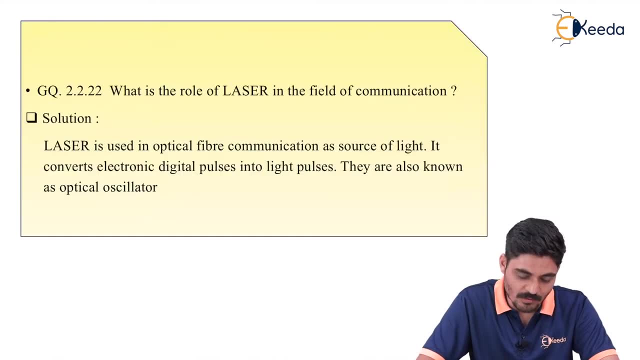 there is use of holography 3. It is used in cutting and drilling of hard metals and diamonds, and it is used in electronic communication. What is the role of laser in the field of communication? because this holography is also constructed using laser. 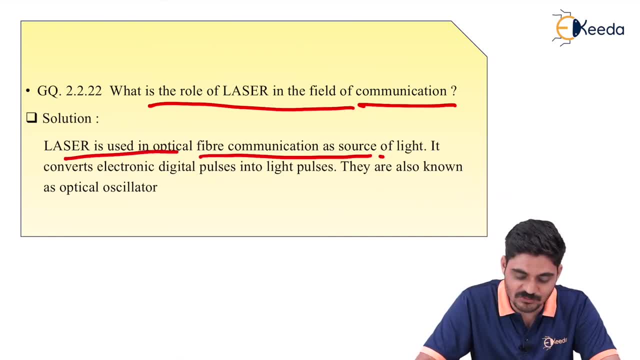 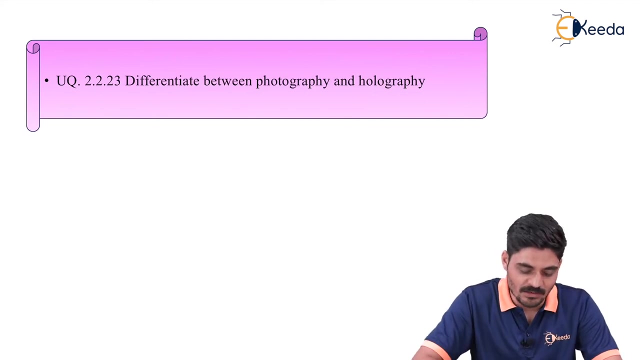 So laser is used in optical fiber communication as a source of light and it converts electronic digital pulse into light pulses. they are also known as optical oscillator. So this is entire thing about holography and uses of lasers in optical communication. Now the second question regarding holography is differentiate between photography and holography. 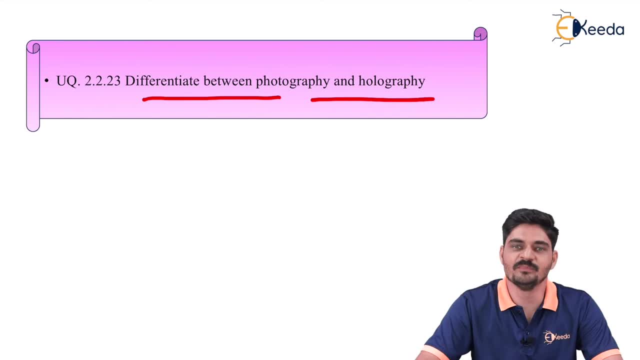 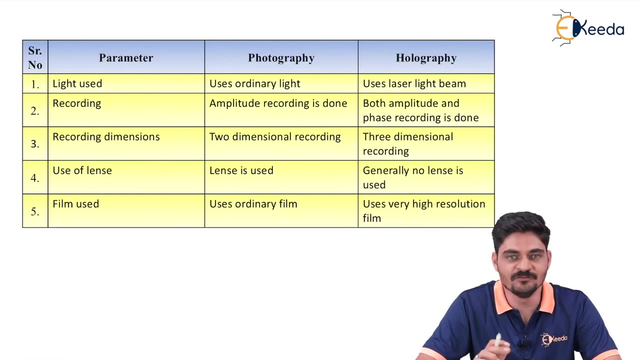 Although it is hard to differentiate, although it is less important, but it is based on holography, which is most important topic. hence you must focus on this question also. so, while differentiating between photography and holography, we will be using few of the parameters, like the light used in photography and light using 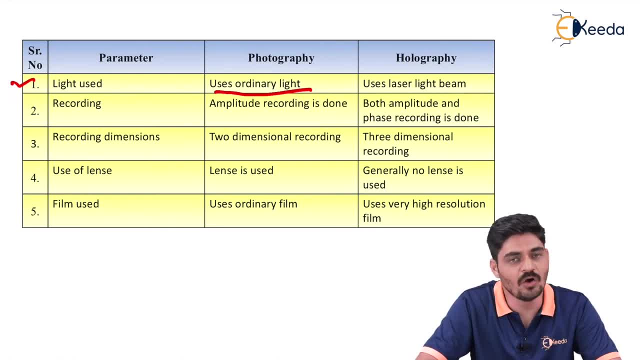 holography. obviously photography uses ordinary light, but holography uses laser light beam and ordinary light also. the second parameter is regarding recording. so in photography only amplitude recording is done. you can say intensity recording is done, as intensity is always directly proportional to square of amplitude. it means if you are recording 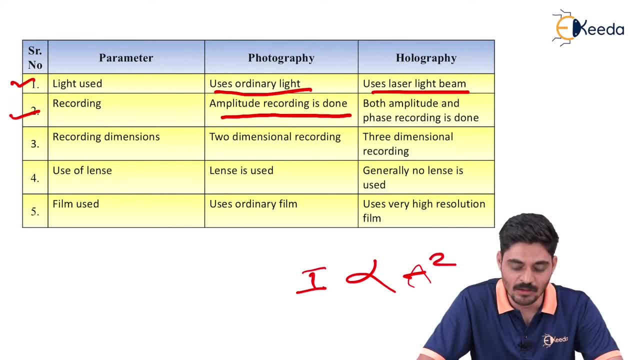 amplitude. you are recording intensity structure, but in holography both the amplitude and phase recording is done. so. in photography, only amplitude recording is done so in holography, both the amplitude and phase recording is done, as i discussed, in holography. the third parameter is: 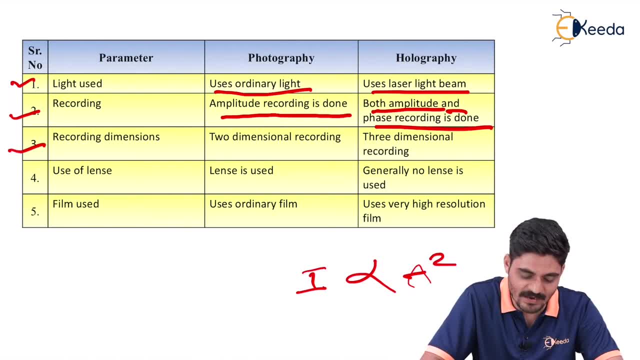 recording dimensions that the photography has two-dimensional recording only and holography has three-dimensional recording and most of the times if you observe holograms on a few objects, if you look at different angles, it shows you 3d diagram of the object. this is not possible. 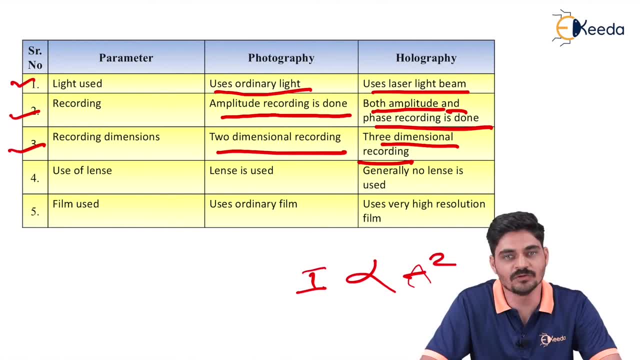 in normal photograph, because in photograph holygrap- there is 2-dimensional imaging and in holograph there is three-dimensional image. what is the use of lens in the photography and holography? in photography lens is used and in holography, as we saw in the diagram of holography construction. 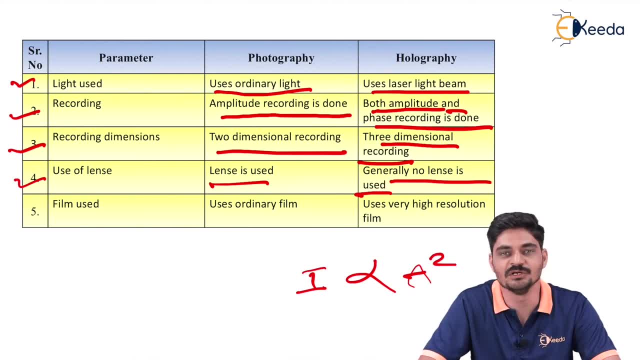 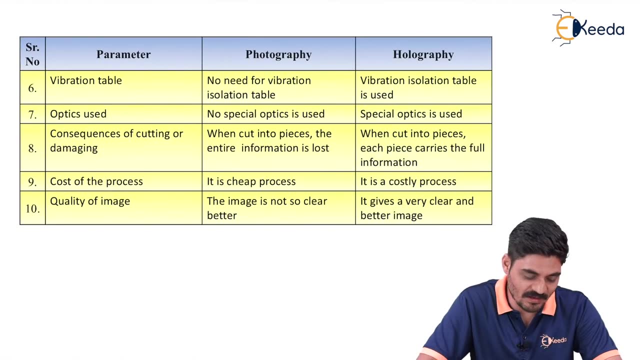 there is no use of lens, so generally no lens is used in holography. which type of film is used for photography? ordinary film is used, but for holography it requires a very high resolution film. the next parameter is vibration table. so in photography no vibrations should be there, so there is no need of vibration isolation table. but in holography.